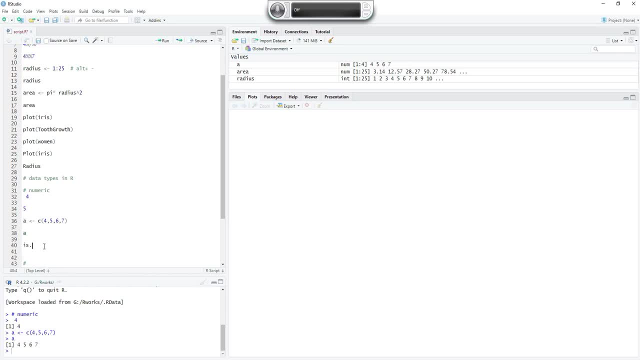 Now we will ask it a question: Is dot numeric? a Argument will be a Run that: Yes, It is a numeric. Now another question: In numeric two types are there: Integer and double. Is dot integer a? Instead of dot I have put comma. Therefore this error is there. I will put dot there. Run that. No, it is not integer, It is four. 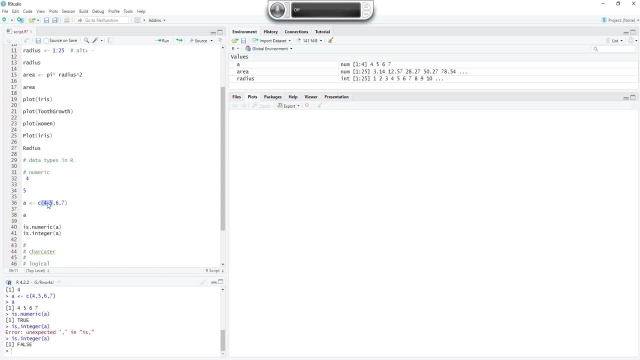 false. We have written whole numbers here, integers here, but R is not accepting it as integer. We will see why. Then is dot double? This is number with decimal points or continuous numbers Run. that Yeah, it is double. R has accepted as double. Now I will do a little. 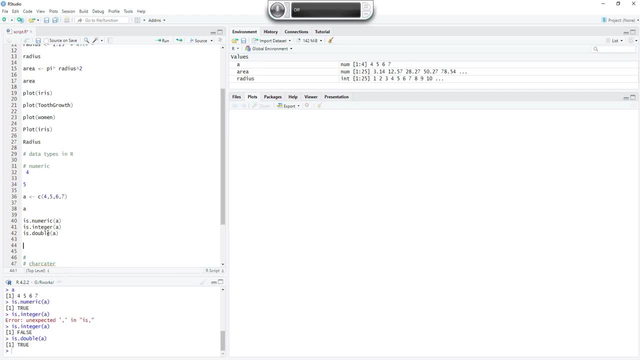 change in that I will declare a vector B assignment operator, that combination and the bracket In this. I will type 4 followed by uppercase L, 5 followed by uppercase L, 6 followed by uppercase L and 7 followed by uppercase L and will run that. Now we will see. 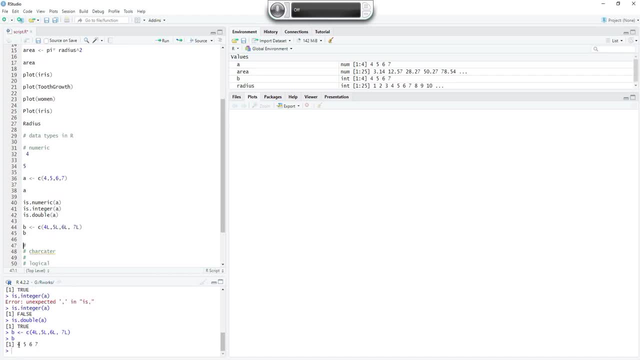 what is there in B Again. B contains 4,, 5,, 6,, 7, but at the back end, R is understanding that it is double. Now we will see what is there in B Again. B contains 4,, 5,, 6,, 7,. 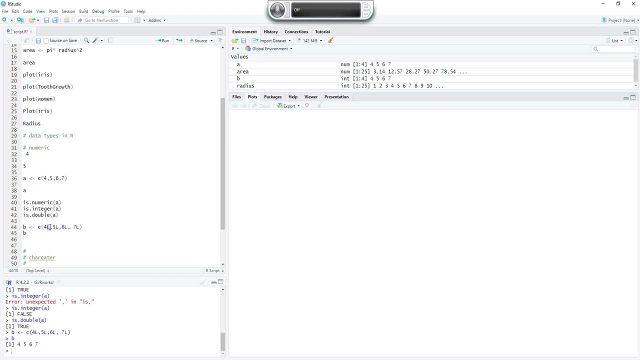 those as integers, because to make those integers, to tell R that these are integers, we have added this uppercase L here. Now we will again ask the same questions: Is dot numeric B? Yes, it is numeric. Is dot double B- No, it is not double. Then what it is Is dot. 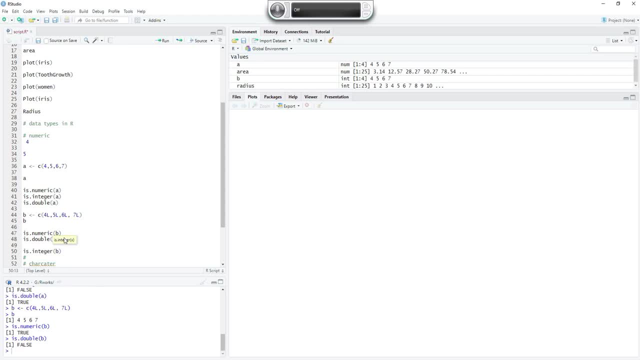 integer B. Yes, it is integer. Why these different data types are there? As you go on practicing R, using R, you will find that the difference between double and integer can be significant for some analysis. Then I will go for the character data. As you have seen how this data 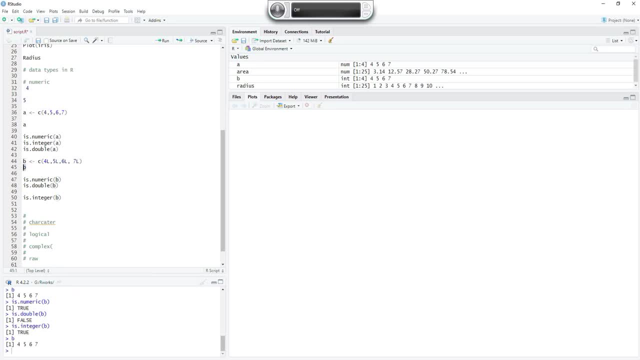 gets printed B. you do not have the inverted quotes here, but for character data this will have inverted quotes. I will type A character and run that C assignment operator C: inverted quote 4, inverted quote 5, inverted quote 6.. Even if this is the numeric data, 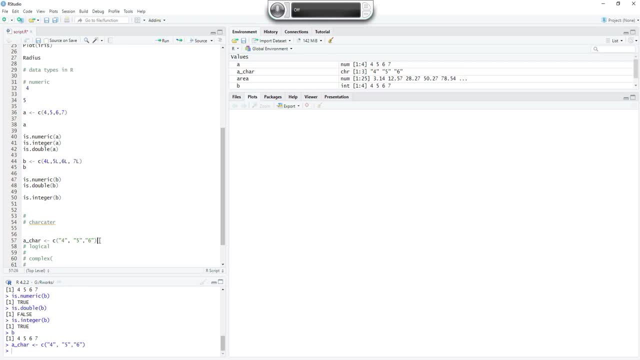 it appears as numeric data, but this inverted quote will make it a character data. Again, we will ask: is dot numeric A underscore character? No, it is not numeric, It is false. Is dot character? Spelling is wrong. And here help is there, I will. 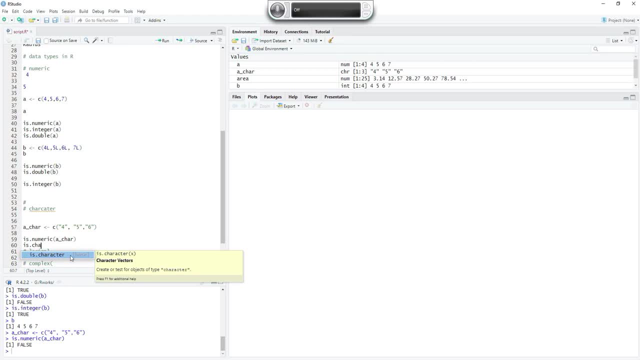 press tab on my keyboard to get the command completed. This is a very good shortcut. Is dot character And there I will type A underscore char Again. tooltip help is there. Again, I will type tab on my keyboard to make it easy for me And this increases my output. 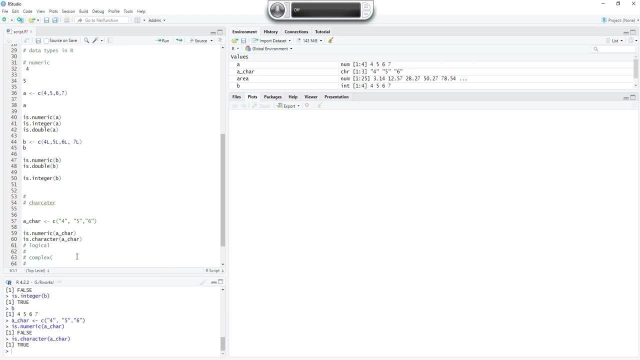 increases speed of my work. Run, that Is dot character. Yes, it is character data. True Character data holds names, numbers and all those I will type here: students, students, that assignment And we will type name of students. 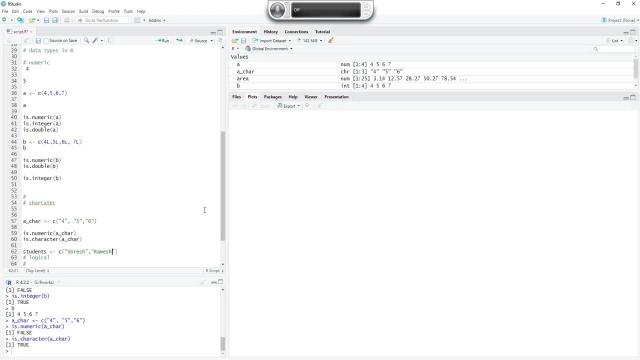 there, Suresh Ramesh, and run that And we will see what is there in the students. Again, you can see that this is character data. Therefore, those inverted quotes will be there. It is not integer data, It is not numeric data or not double. You can add any number. 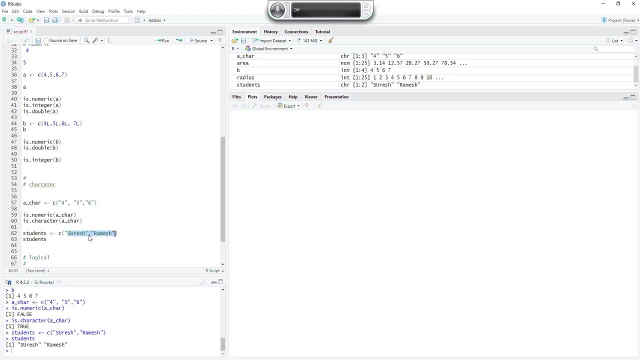 of values in this vector. This is character data. I said Then we will go for For the logical data: A- logical- I will type there A underscore- logical assignment operator. and C- Logical data contains these values. True, All caps. Always remember that this. 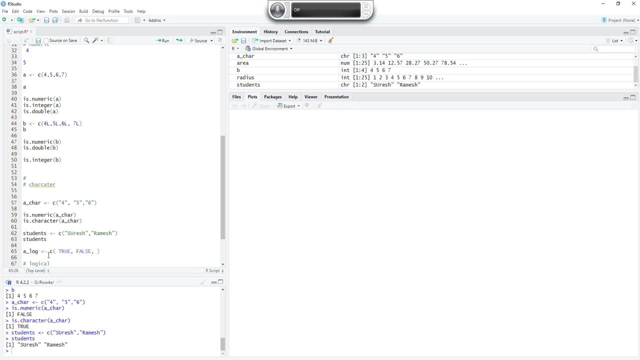 is all caps, False Again, true, True. Only these two values will be there. Therefore, this type of data is also called as Boolean data- I will give the name logical here, because I have not Not worked here- And complex and raw. we are not going to discuss This, I will run Control. 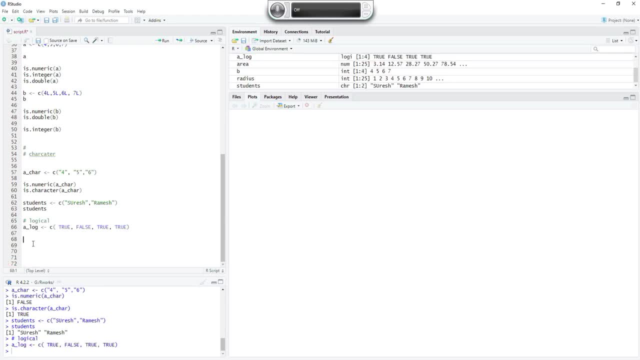 enter And we will ask it to print A underscore logical And run that It is saying true, false, true, true. Now you can see these values are getting printed in different color. These character values are also getting printed in different color And numeric values are. 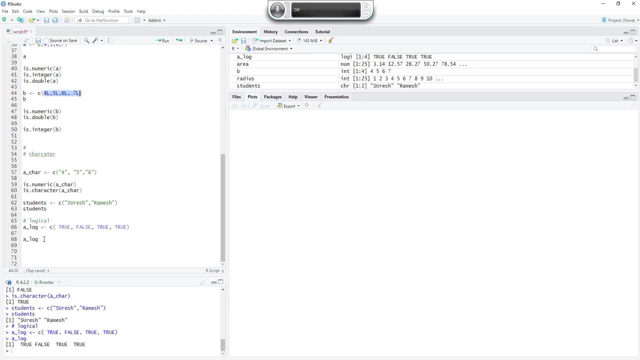 also showing in different color. So you need to know what the value is. get the value of the values down And suit these here. We pray that we don't mess up your code highlighting- code highlighting to help you understand what type of data it is Highlighting. you can change, But if you are familiar with this, 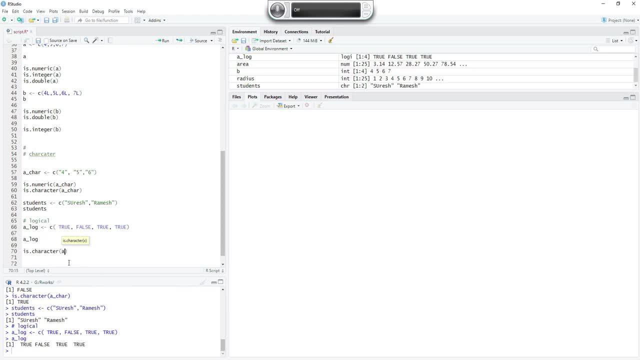 colors. that makes you Makes handling your data very easy. We'll ask it question: is dot character A underscore? log And run that? no, it's not numeric. is dot logical? a underscore log and run that? yeah, it's true, it's logical data. 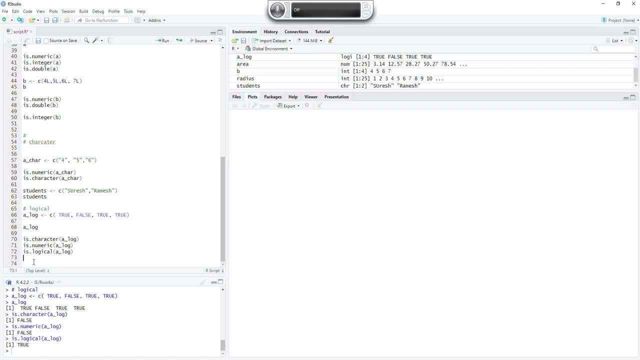 those complex data and raw data we require very less number of times. therefore, i will not discuss that uh. in next session we'll see how to uh interconvert this data, how to convert character data to numeric. what happens if we convert that then? how to convert numeric data to character. 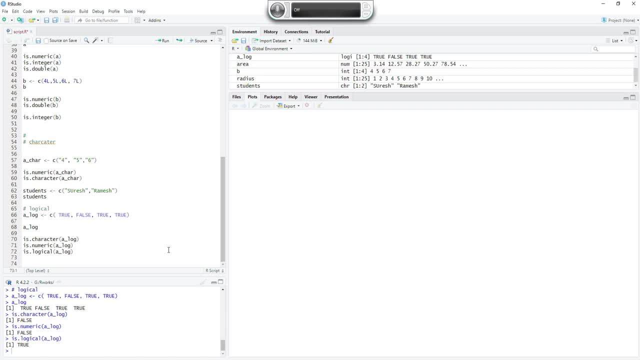 we'll see what happens then. then, logical to numeric, logical to character, we'll see how that data can be interconverted in between and we'll see data coercion also. that's a very important concept to learn about data types. that's all for this session. if you like this video. 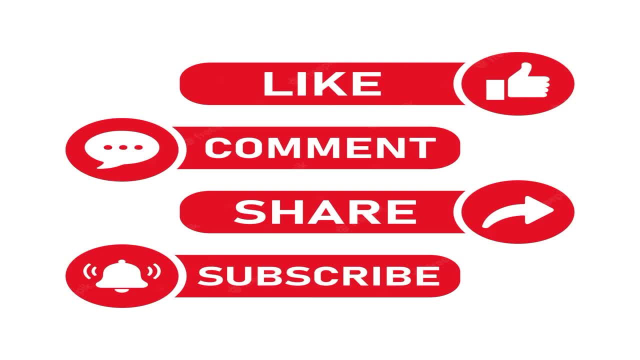 please click like button. share this video with your friends, subscribe to my channel if you are not subscribed yet, and press the bell icon to get notification of my new videos. thanks, thanks for watching this. 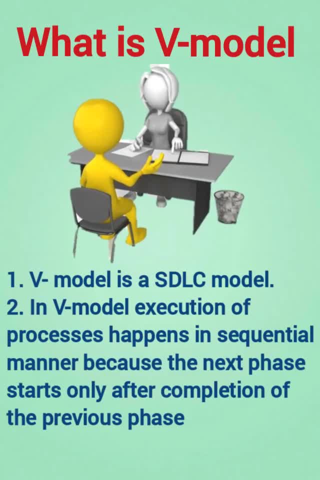 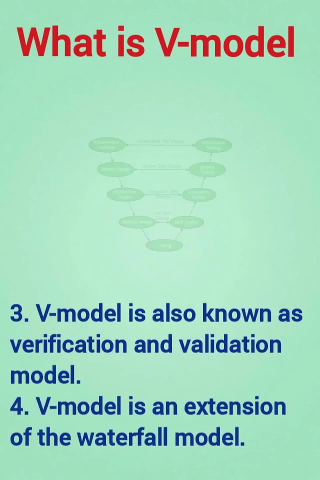 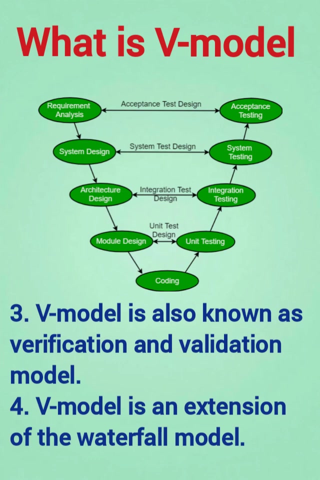 Software testing interview questions. What is V model? Answer is: first: V model is a SDLC model. Second, in V model, execution of processes happens in sequential manner because next phase starts only after completion of the previous phase. Third, V model is also known as verification and validation model. Fourth, V model is an extension of the waterfall model. Fifth, in V model, each development phase associated with the testing phase in reverse manner.